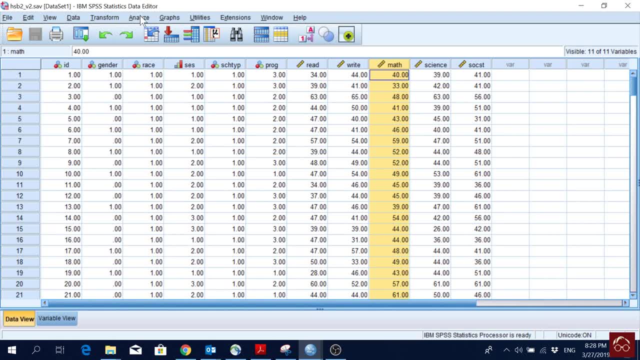 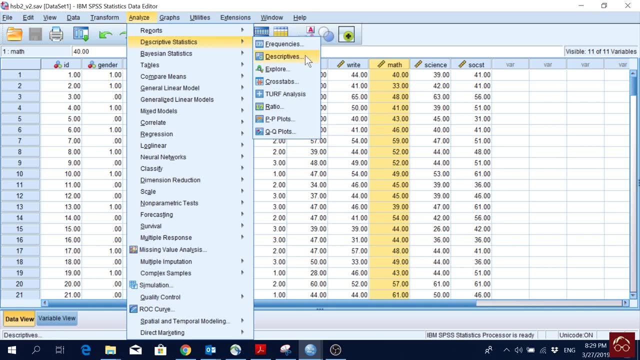 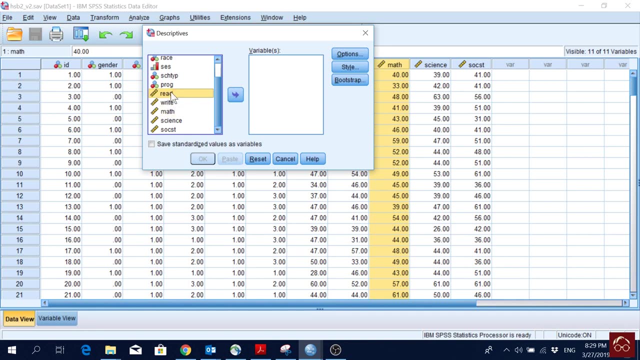 the previous previous video. okay, so for descriptives, we'll go to analyze, we'll go to descriptive statistics and we'll go here descriptives. okay, so we will click it and i will drag all my variables, all my variables of interest. so i will click the first one and then. 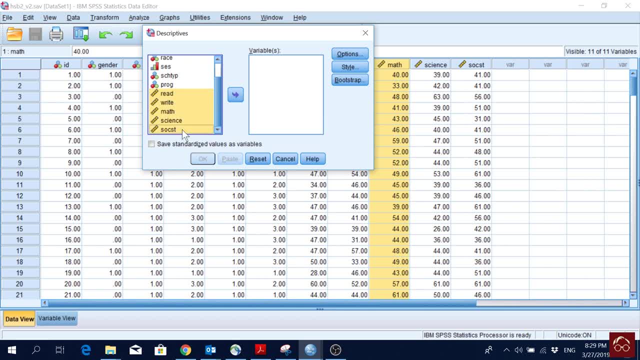 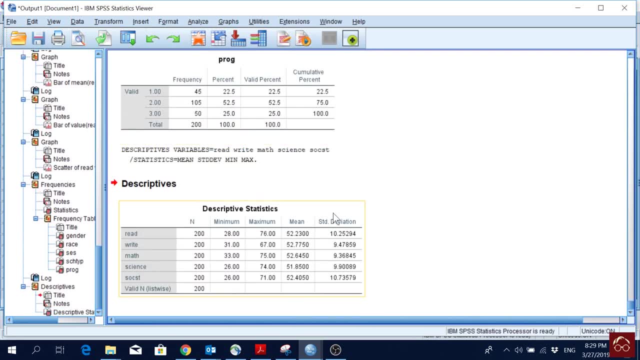 the last and and then i will press shift and i'll click the last one. all of them are selected. i'll move them here and then i will click. ok. so this is the by default descriptive statistics that i get: the number of observation for all the variables, the minimum values in each of them, the maximum. 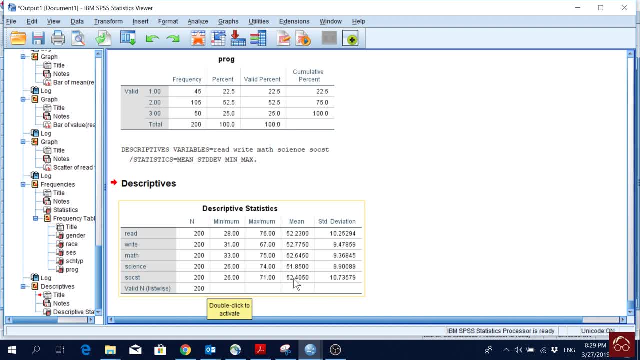 values in each of them, the mean score for all the continuous variables and their standard deviation. but sometimes, you know, we want to see even more. we want to see the standard errors, we want to see this code. yeah, we want to see the skewness scores and cartosys scores. 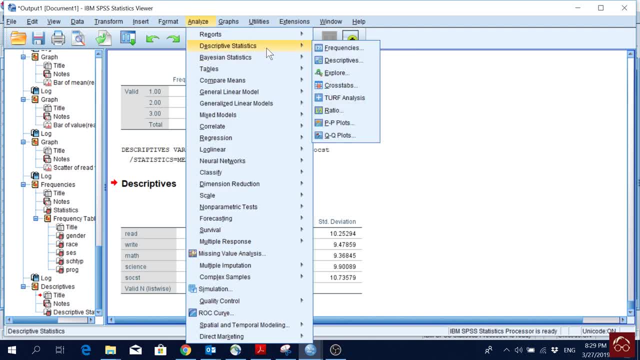 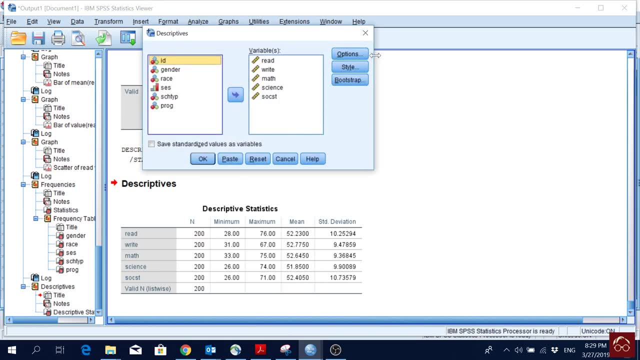 to to have those values. i will go to analyze, i'll go to statistics- descriptive statistics, then descriptives, and then i have the same setup. okay, i'll go to options. then i can actually choose what else i want. i want variance, i want range, i want a standard error of the mean. 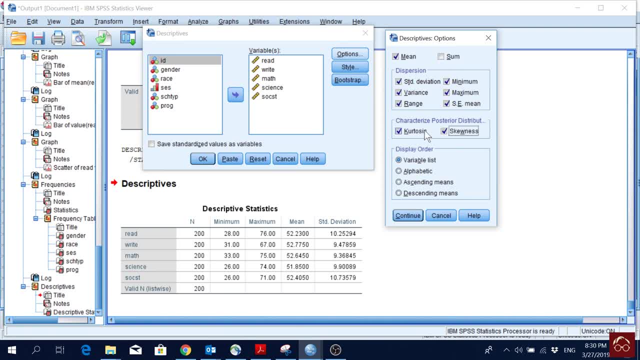 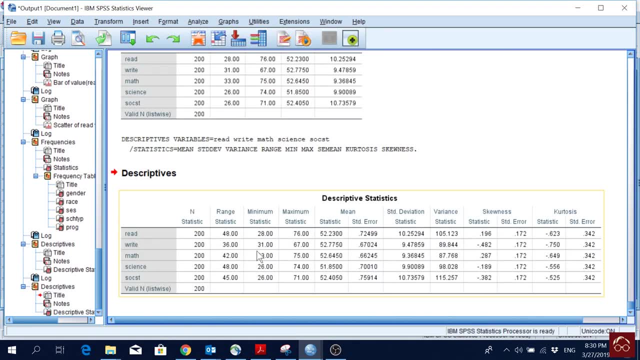 skewness. okay, so i want all of it and, yeah, i'll click continue and i'll click ok. so now you see that we have a broader descriptive statistics table. okay, the number of observation range: statistic. what is range? the difference between the smallest and the largest value in. 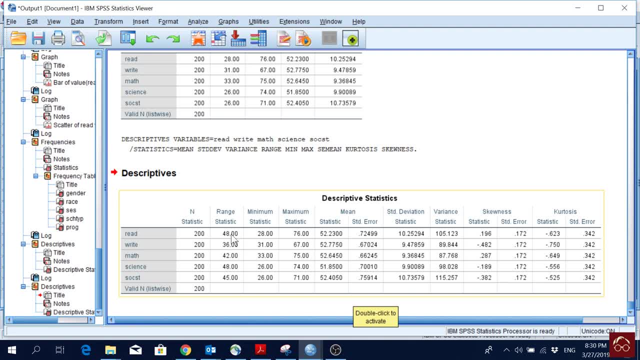 our data set. so the difference between 28 and 76, that is 48.. then we have the mean of mean, mean of the standard error and the standard deviation. so we have all the variables here and their respective standard error. okay, how is the standard error calculated? the standard error is: 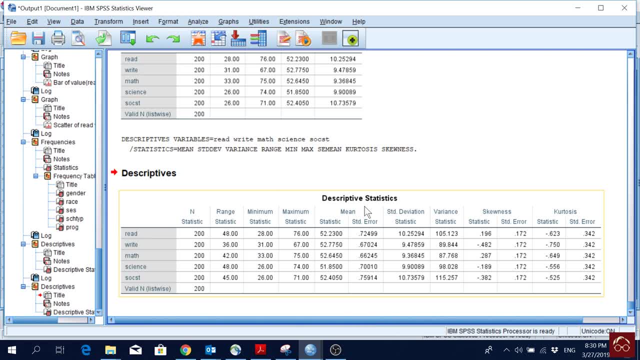 the standard deviation divided by the square root of the number of observation. okay, that's how we get the standard error. it reflects how our sample mean is different from the population mean. that's what we get from a standard error. the smaller the small. the smaller the standard error, the closer our 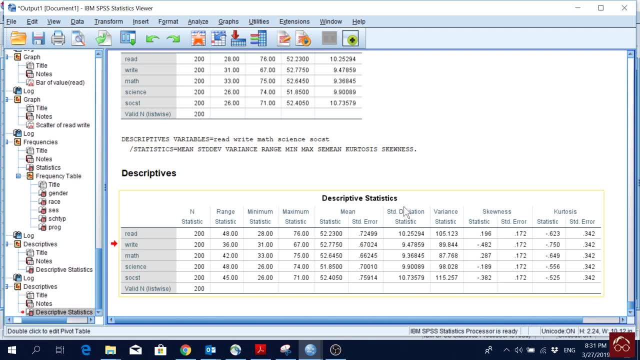 mean. and then we have the standard deviation statistic, we have the variance, and then we have the skewness and we have the kurtosis, okay, and we have the skewness scores and their standard error, kurtosis scores and their standard error. as you see, that for a normal distribution, we, as I, if you remember, in 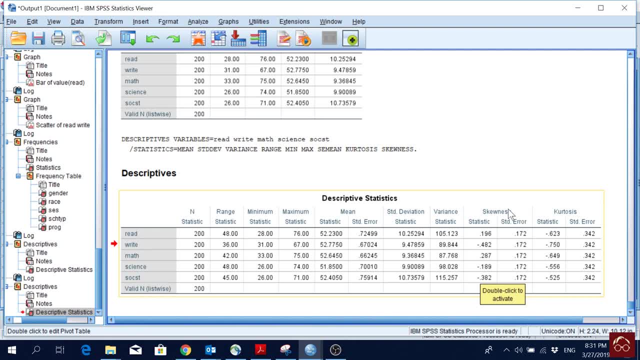 the previous video I said that for a standard deviation we will need a skewness value of zero and kurtosis value of three. both of them together okay. but in this case we see that although our skewness values are not zero, but they're close to zero, okay. I also say that we can have a range of plus one. 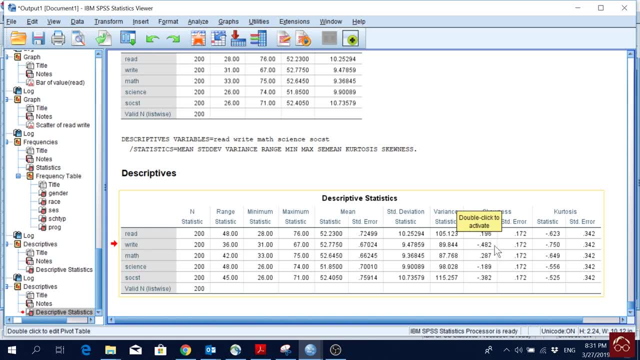 and minus one, and actually we see that the skewness values are within a range of plus one and minus one, so they are rather okay, but kurtosis values are far from three okay and that means that the data most probably is not normally distributed. but we cannot still conclude if we want. 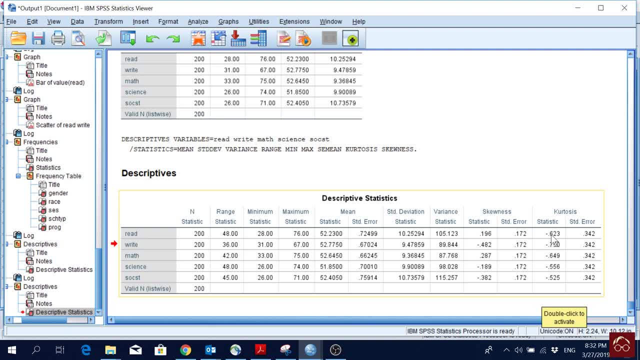 to conclude that we have a skewness value of three and we have a range of six. so let's conclude: if data is normally, skewness values are within a range of six and we have a range of six. so let's see our video on how to check normal distribution and then you will see in. 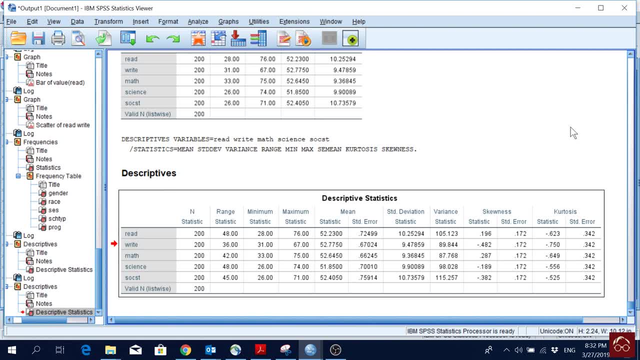 detail how we check for normal distribution. so that's what actually we can do for on descriptives, and these are the major descriptives that we normally present in a research paper, and thank you for watching this video. if you like this, please comment, share and subscribe to your youtube channel.